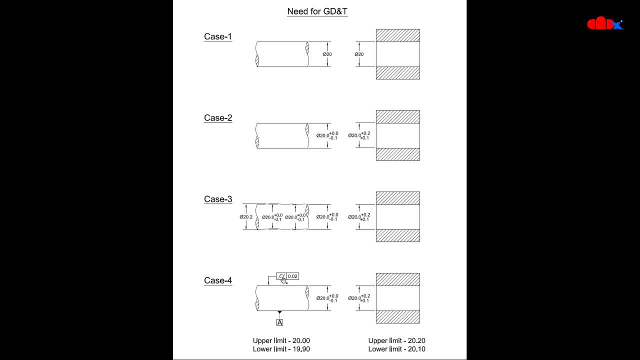 These dimensions are the general dimensioning and tolerancing And if you see this dimension, this is geometric dimensioning and tolerancing. So again, the general dimensioning and tolerancing control the size of the part and GD&T control the shape of the part. 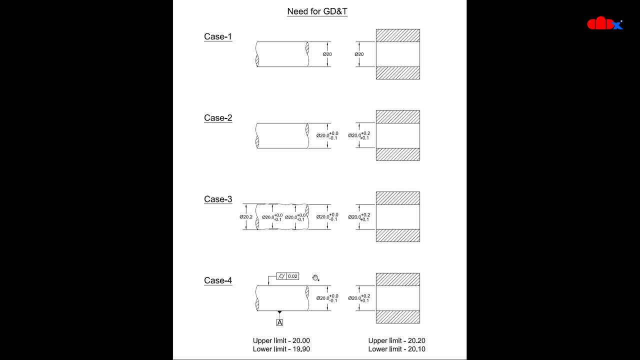 Now let's understand the need of GD&T, and by this practice you will further understand the difference between these two. So let's start with case 1.. So here, as a design engineer, I designed these two parts with a die at 20-20 and I sent it for manufacturing. 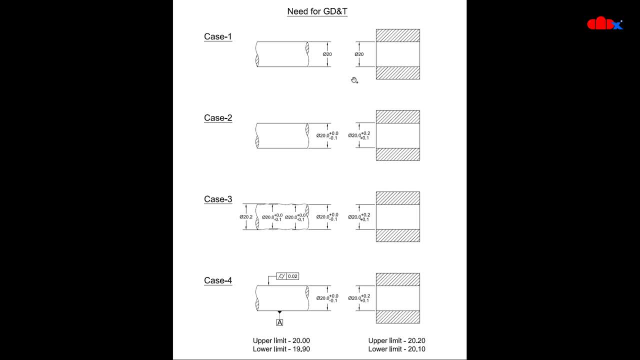 And I asked the manufacturing guy to manufacture 10-10 components each. But when I received it I found that I was not able to assemble any of this shaft with the hole. Then again, I cross checked my drawing and I found that both dies are 20-20 and there is no enough clearance to assemble it. 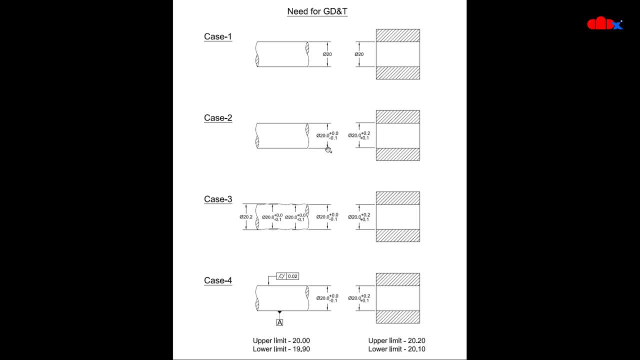 So I corrected this drawing and made this drawing like this. I added tolerance here. So now, in this case, if you calculate upper limit and lower limit, you will find that the shaft die is always smaller than the hole die, So it will go inside easily. 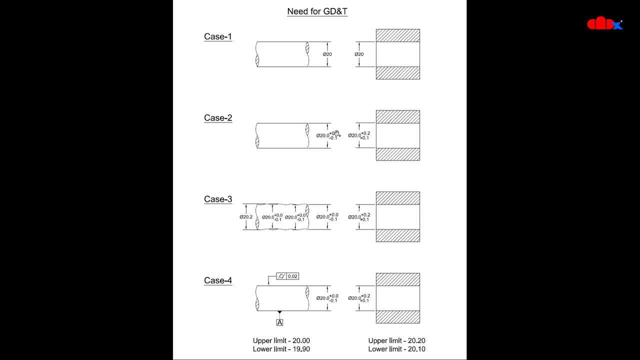 So here, if you calculate this upper limit, 20 plus 0 is 20 and lower limit is 20 minus 0.1 is 19.9.. So it is 20 and 19.9.. And if you calculate this upper limit and lower limit, the upper limit is 20.2 and the lower limit is 20.1.. 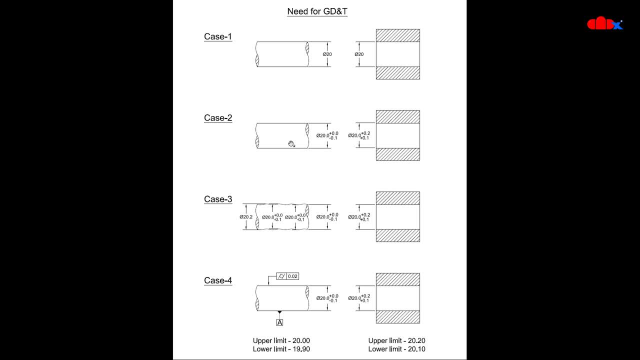 So here the smaller hole is 20.1.. And here the bigger shaft is 20.. So in all cases I was having enough clearance to insert this shaft. So after this modification once again I sent this drawing to the manufacturing guy And again I asked to manufacture 10-10 components. 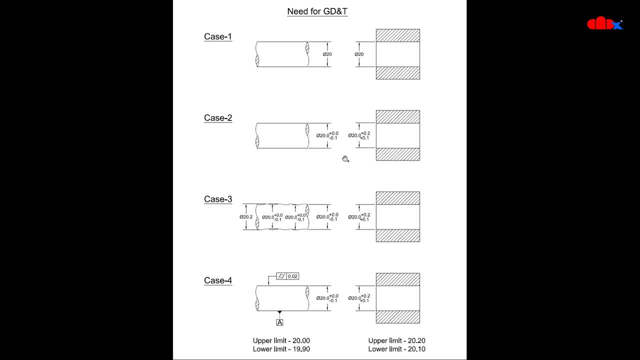 When I received these components and I tried to assemble it, I found that I was able to assemble almost 70% of the component, But still 30% of the component was failing. Now once again, I rechecked these drawings to find the error. 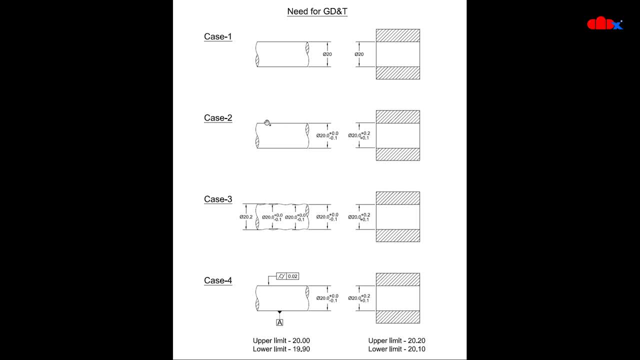 And I found that When I zoomed this top surface of this shaft, There was some deviation like this. So when I checked this dimension in multiple sections, I found that my dimensions are correct in each section, But still it was not going inside. 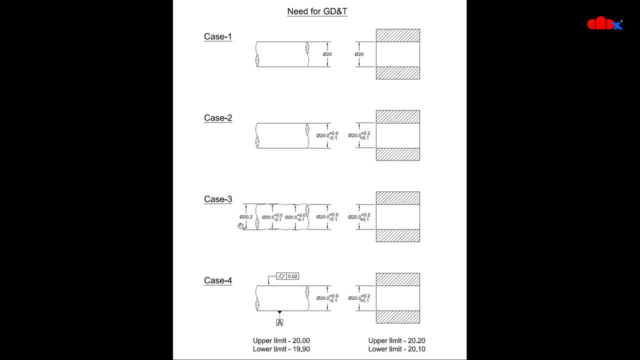 So when I checked the overall outer to outer dimension I found that this is bigger than the lower limit of the hole. So when shaft die is bigger and the hole die is smaller, It will not go inside. So in 30% of the shaft cases 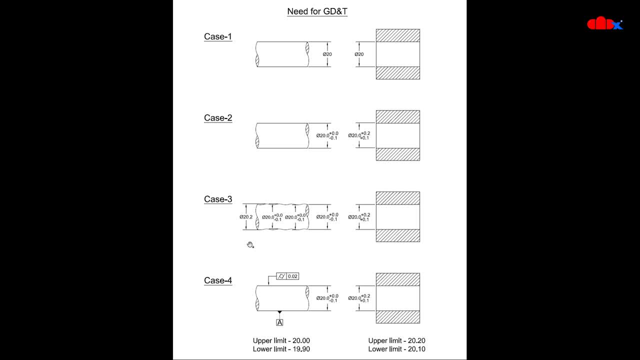 The outer to outer die was bigger than the hole die. So now I understood the problem: That my size is correct But my shape is incorrect. So to correct it, I was not having any option By general dimensioning and tolerancing, So I adopted one method which is called geometric dimensioning and tolerancing. 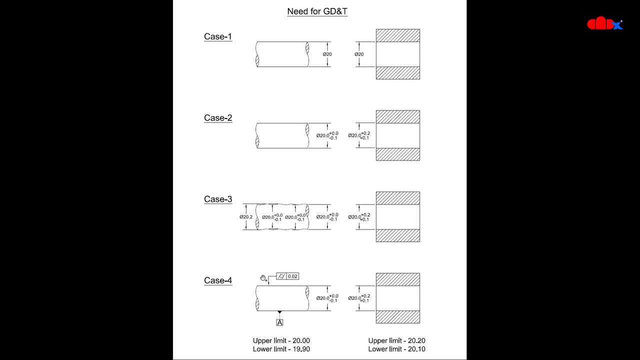 Now, to control this deviation, I implemented one symbol with tolerance value. So now, in this case, if you see, The deviation is 0.2 with nominal die 20.. So here the deviation is 0.2.. So to control that deviation, 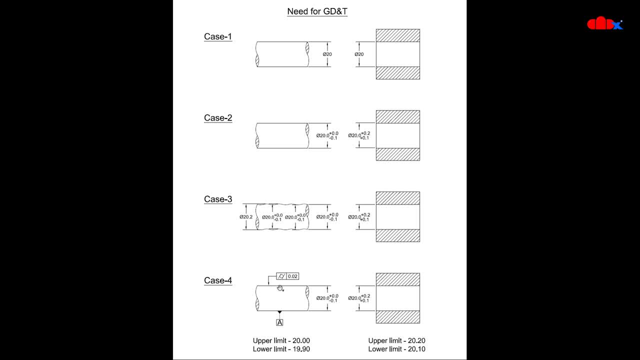 I added cylindricity with a tolerance value 0.02.. So here I am telling that the maximum deviation of this surface Should be within this range, 0.02, not 0.2.. So now, in this case, Your upper limit of the shaft is 20.. 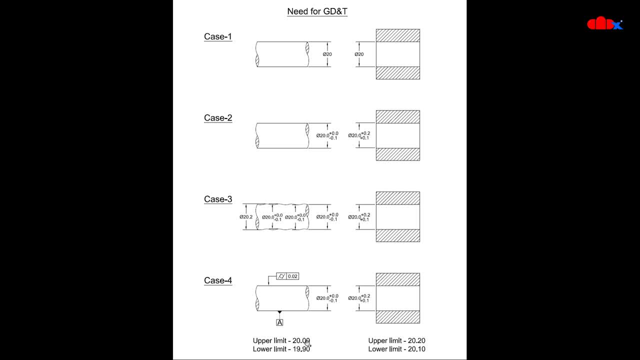 That means the bigger die of the shaft is 20.. And if you have this deviation, 0.02.. Biggest die of your shaft will be 20.02.. And if you come to The smallest die of your hole, It is 20.1.. 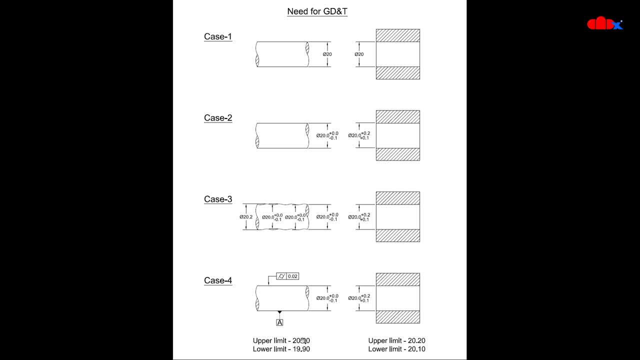 So still, the smaller die of the hole Is bigger than the bigger die of the shaft, So in that case It will fit easily. So when I sent this drawing for manufacturing And I received the component This time I found that My all 10 components were fitting correctly. 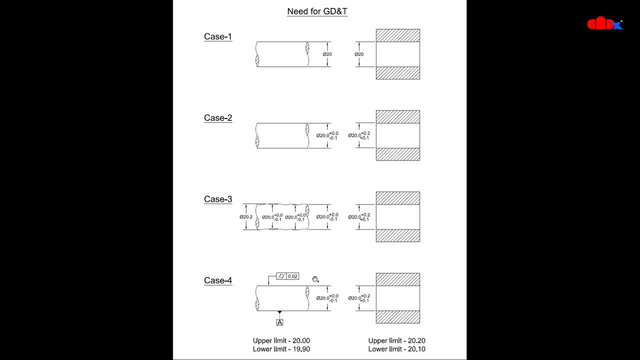 And that is how We understand the importance of GD&T. So now in case 4.. I have general dimensioning and tolerancing With GD&T. So when you implement GD&T, You minimize your rejection And you correct all your components. 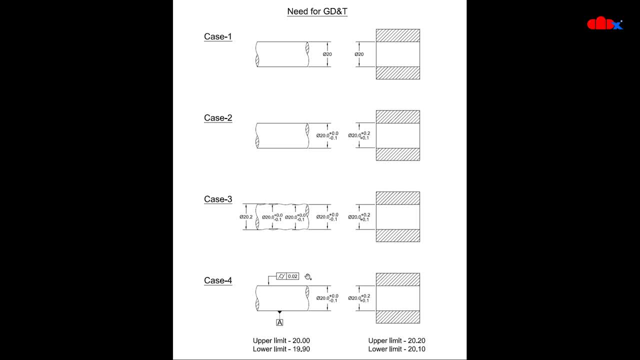 So now you understood the need of GD&T And you are much familiar Between general dimensioning and tolerancing And geometric dimensioning and tolerancing. So this was the first part. Now let's move to the second part, Where we will understand. 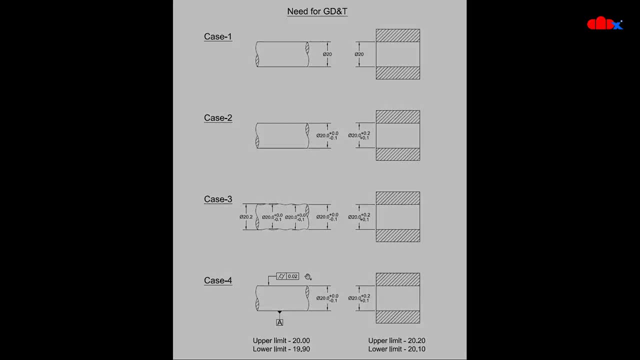 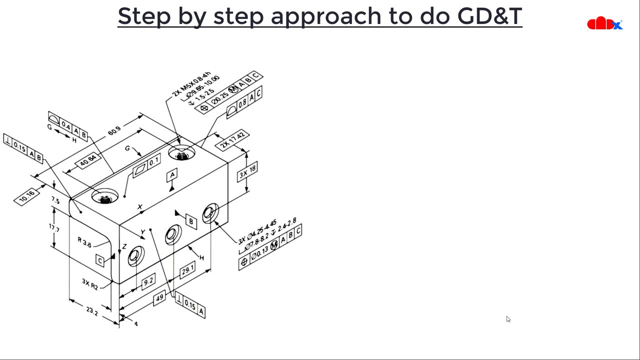 The step by step approach To do GD&T. So before I start the second part, Let's understand some basics about GD&T. So the GD&T Stand for The geometric dimensioning and tolerancing, And there are multiple levels of GD&T. 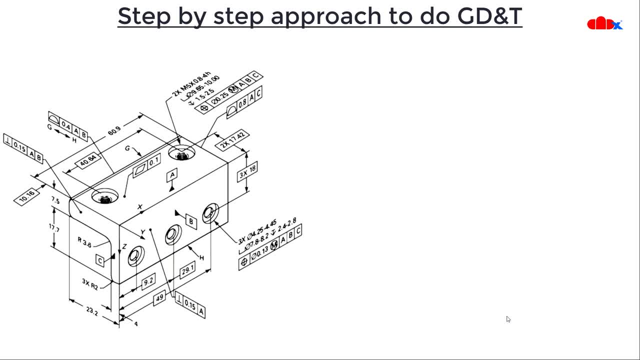 Like level 1., Level 2., Level 3. And so on. But as the level of GD&T increases, The manufacturing cost also increases. So we all avoid multiple level of GD&T. We try to minimize it. So when we do GD&T for any part, 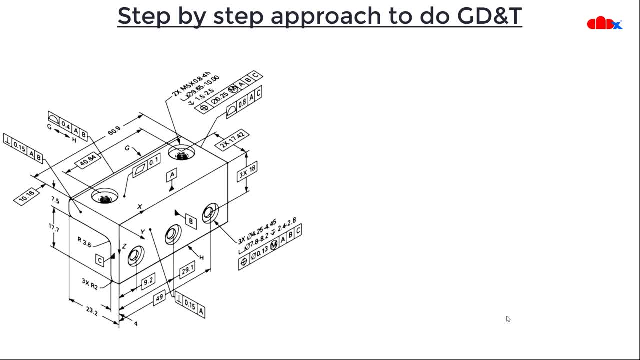 There must be a physical relation For that particular part To another part Inside the assembly. So if there is no assembly, There is no GD&T. So let us assume that You have a individual component Which itself is a complete product. 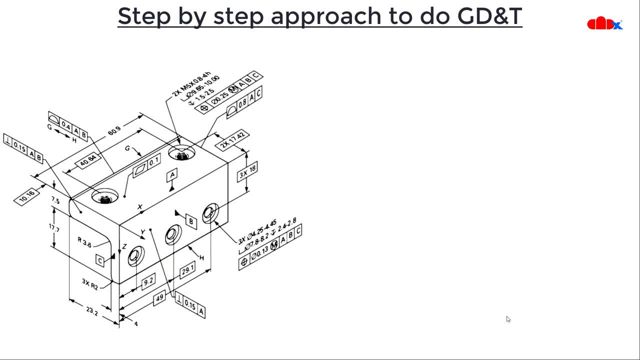 Then there is no GD&T. Your general dimensioning and tolerancing is Good enough To manufacture it. So now you understood That whenever we do GD&T, That means There is a relation For that particular part To another part. 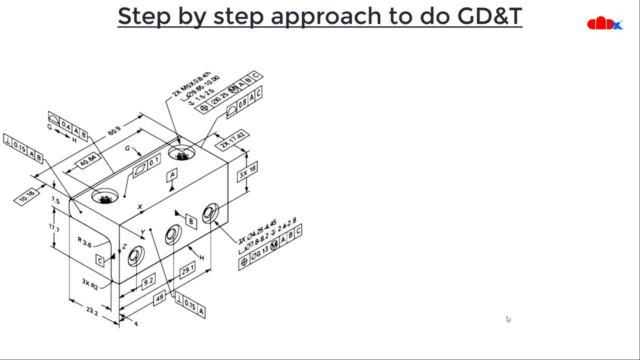 Inside the assembly. Now let's understand The step by step approach To do GD&T. So the first thing is, When you start GD&T For any particular part, You need to place The 2D views in your drawing. 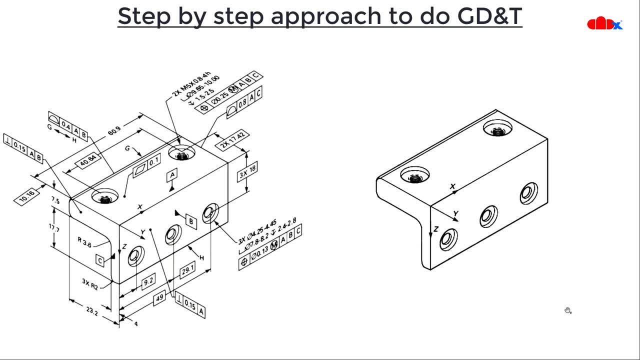 So let us place the 2D views. So I place my 2D views here. So in my case, I have placed a 3D view For better understanding. So you will be placing 2D views In your drawing. 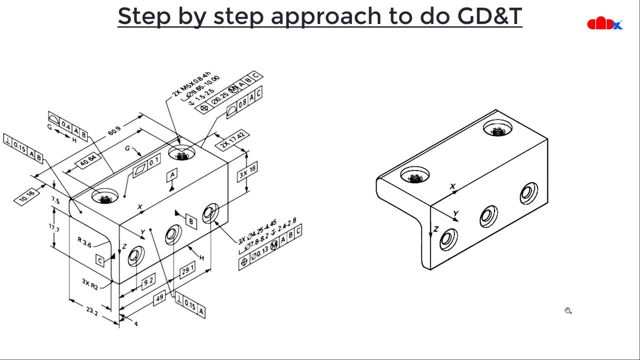 So, once 2D view is placed, Now you need to decide That which surface You are going to place On the inspection table. Now, let us assume that This is the surface, The top surface, I am going to place. 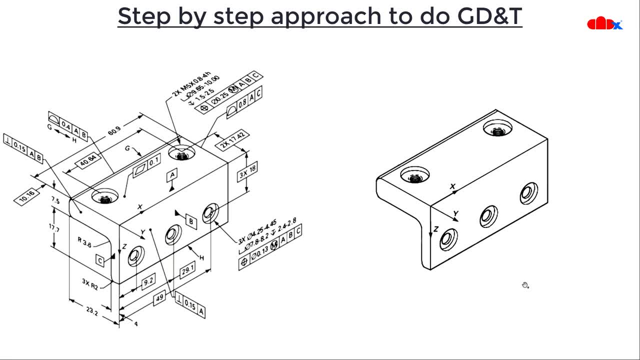 Onto the inspection table. So the moment You decide One surface To be placed On the inspection table, That surface Has to be The perfect surface Before placing To the inspection table, And that is why We place. 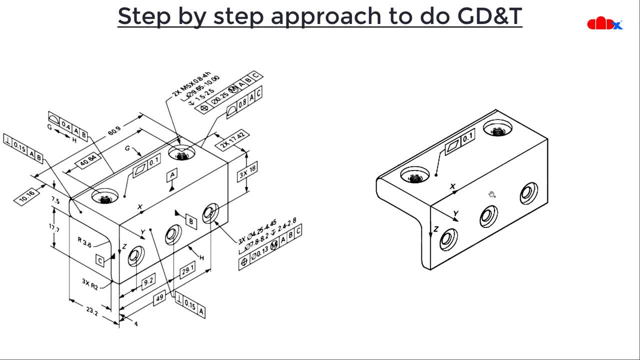 Flatness To that surface. So If you decide This surface To be placed First on the inspection table, Then this surface Will get flatness. But in my case I decided To place This surface Onto the inspection table. 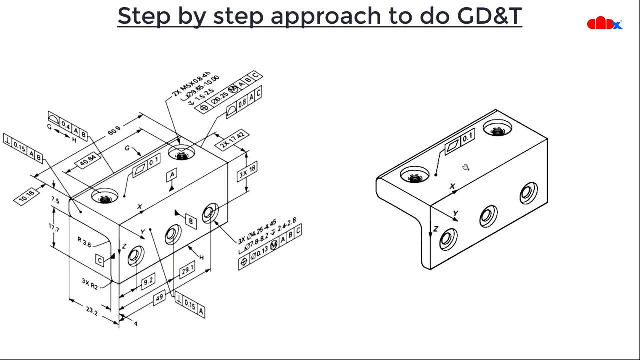 So automatically This surface Will get The flatness, This surface To be completely Flat. You added Flatness. Now, after that, You can consider That surface As your datum A, Because this surface Is the surface. 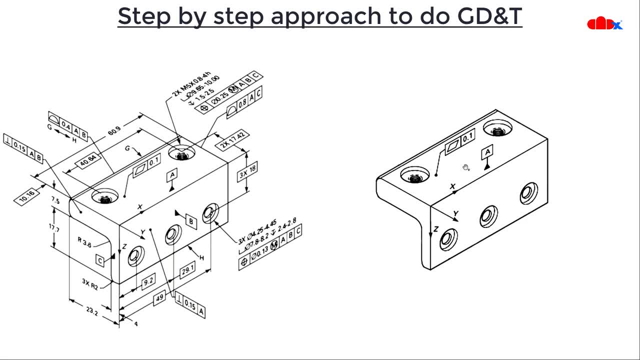 Which is going And sitting On the inspection table And this surface Is completely Perfect And all the dimensions I am going to reference With this surface. Then I can make This surface As datum A. Now my datum A. 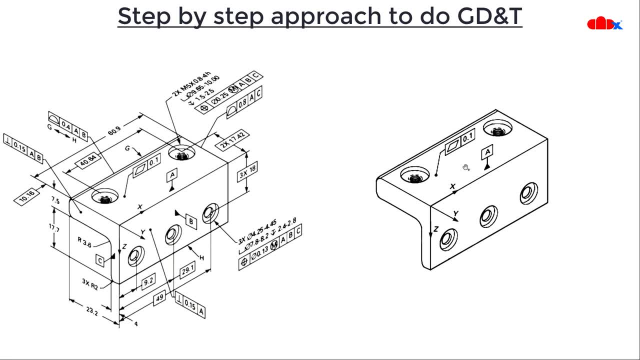 Is decided Now. I can go with Single datum Or multiple datums. As per my requirement, I am going with Multiple datums, So the next step is Decide the datum B And datum C. So I have decided. 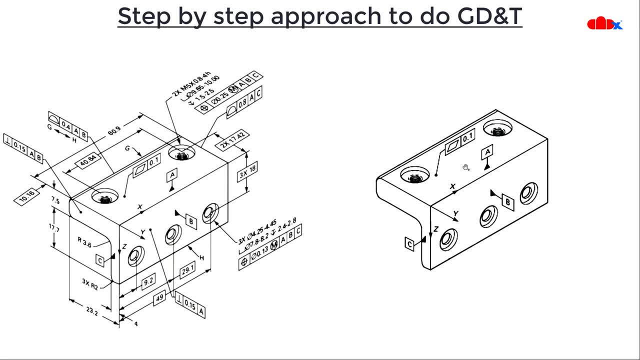 Datum A, B, C. So once you decided All your datums Now, datum A Is your primary datum, Datum B Is your secondary datum And datum C Is your tertiary datum. Now, sometime, You won't see- 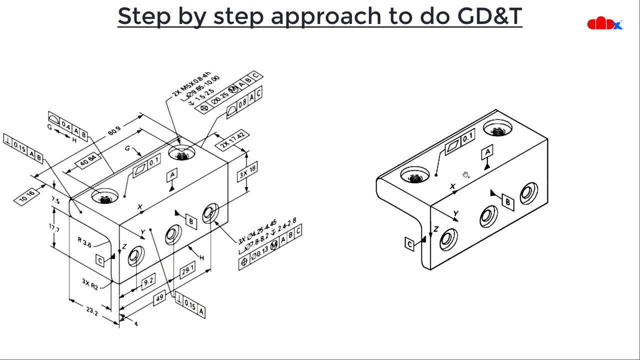 Any flatness Applied to any part. That is because If the size Of the part Is very small, It is coming Within the tool size. Then without applying Flatness also, You get the perfect Surface. So in that case 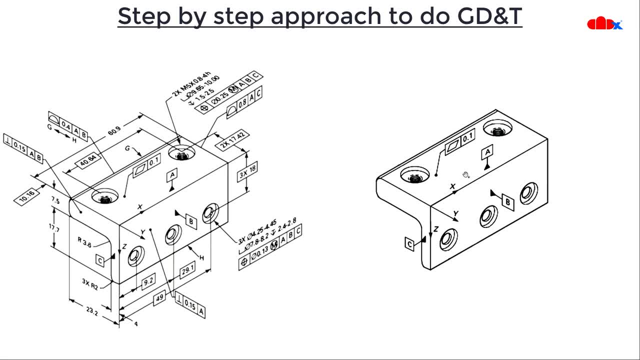 No need to apply Flatness, But if the size Of part is bigger Than your tool size, Then you must apply The flatness. Now, once you decided Datum B And The relevant surface Is also having Some functional, 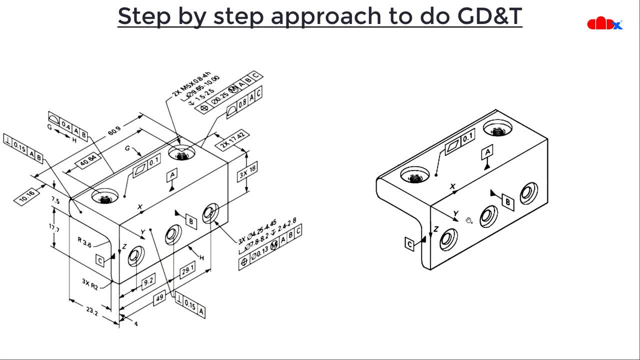 Requirement In the assembly, Then you must apply GD&T For that surface Also. So that is why I have applied GD&T For that surface. Now, this symbol Says Perpendicularity. With this tolerance, You are telling that. 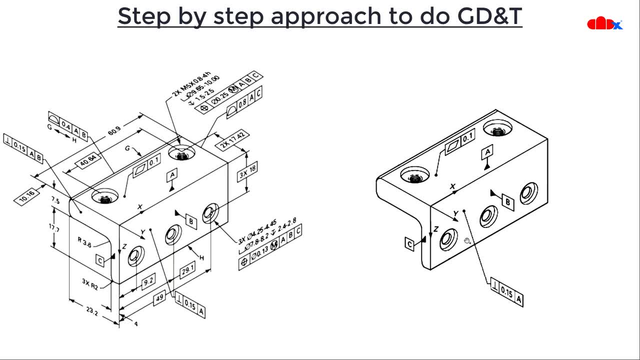 This surface Has to be 90 degree. With what? With reference Of some Other surface, And that surface Is datum A. Now, one more thing You need to understand Here Is when you give This tolerance 0.15.. 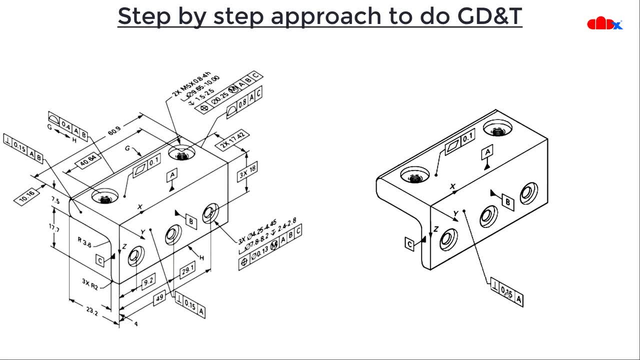 You are telling that The deviation Within this surface, The upper limit And lower limit- Should be Within this range. That means You are again Applying the flatness To this surface. So when you apply Perpendicularity, 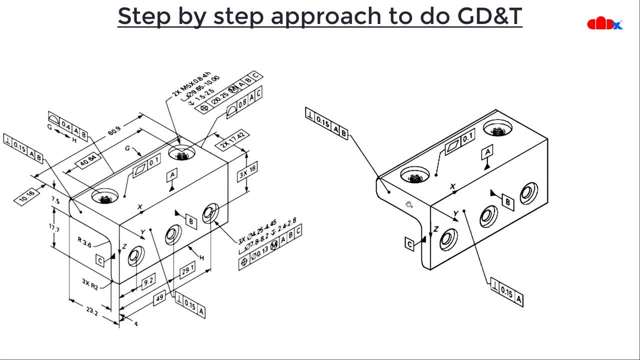 By default The flatness. Then I will go for This surface, GD&T, And here again I have applied Perpendicularity With reference Of A And B, So this surface Has to be 90 degree. 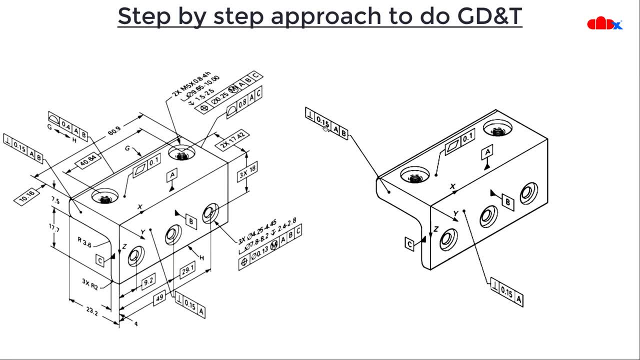 With reference Of this surface Also, And this surface Also, And the deviation Within the surface Should be Within 0.15.. Now, once You have decided The GD&T Of this, Then you will go for. 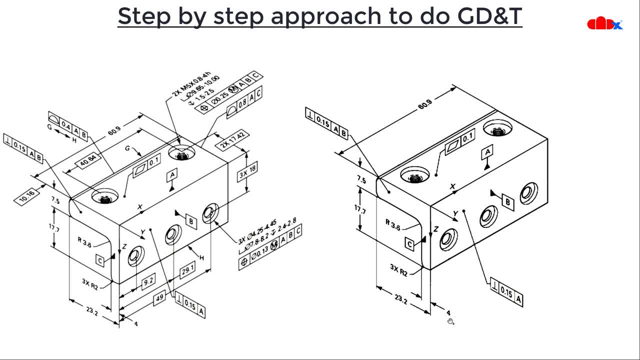 Dimensioning. So these are the Dimensions Of the drawing, Maybe in your Title block Or Somewhere With a note. Now the next step. So in next step We further have Some more dimensions. But You will notice that. 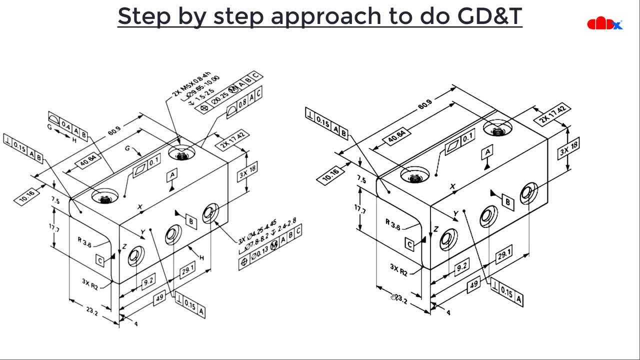 These dimensions Are having one box. So what is Difference between This dimension And this dimension, Or this dimension And this dimension? So there is No difference Between these two Dimensions. The only thing is, When you put: 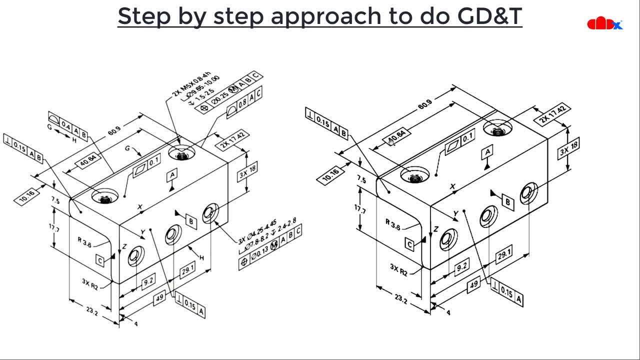 A box With any dimension, You say that This dimension, So the general tolerance Which is applied To this dimension, Is not applied To this dimension. So once you put The box, You are telling that For this particular dimension, 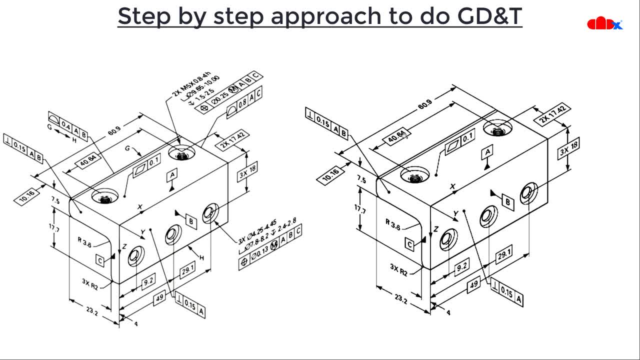 We have a separate Tolerance Written somewhere In the drawing Now, where These tolerance Are written In the drawing That you will understand In next slide. So now This dimension, These two dimensions Are the whole dimension. 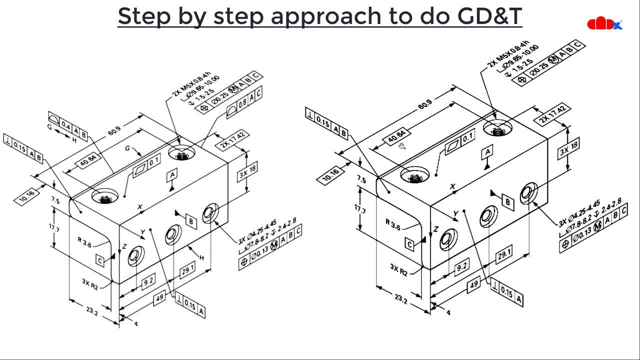 Now, if I move Further, You get Position tolerance. Now let us Look at the Tolerance dimension. You will see This box Covering this dimension. So if you see This position Dimensions Carefully, You will notice that. 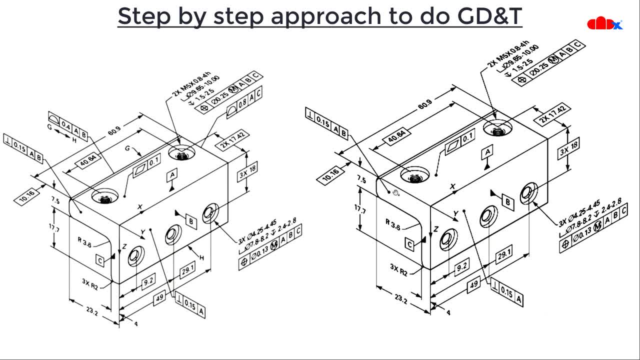 These dimensions Are applied To the center axis. So This dimension Says that The distance From this surface To this center axis Is 10.16.. And the distance From this center axis To this center axis. 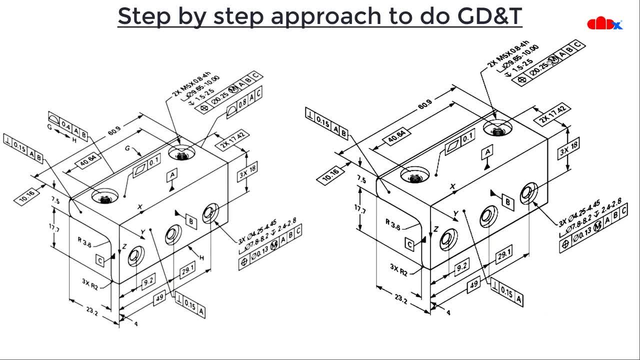 Is 40.64.. So these dimensions Positions The axis Of the whole And if you see The position tolerance, That means That tolerance Is for the center axis If a datum Is attached To the dimension. 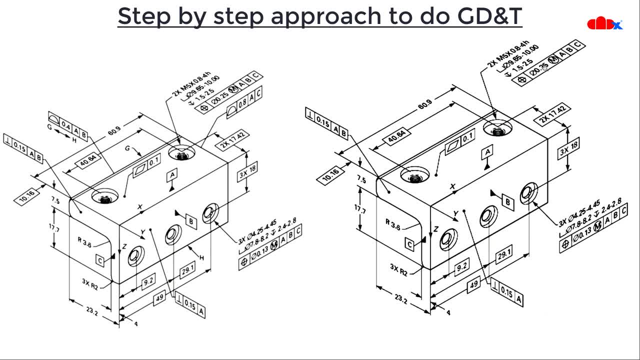 That means The datum Is the center axis. Similarly, If A GDNT Is attached With the dimensioning, It is for The center axis. So now, Here You are telling that The position Of this center axis 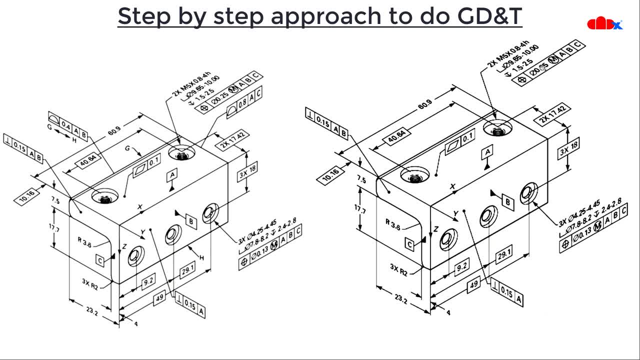 Should be Within this range With reference to The datum, A, B And C. So again, This is the dimension Of the axis And this is the tolerance Of the axis. So for this, Special dimensions, The given tolerance. 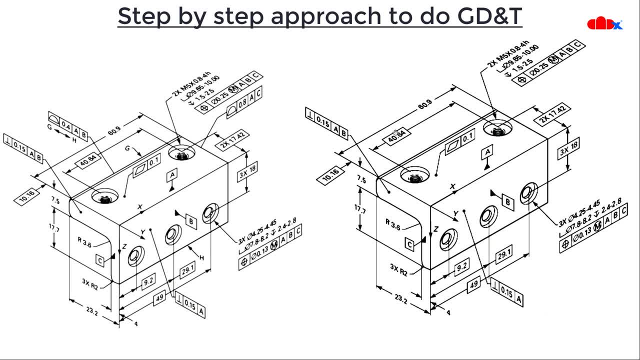 Is here. So this is the tolerance Applied to These dimensions, And that is why The general tolerance Is not applied To these dimensions. So once you complete Your general dimensioning And tolerancing With GDNT, You have completed. 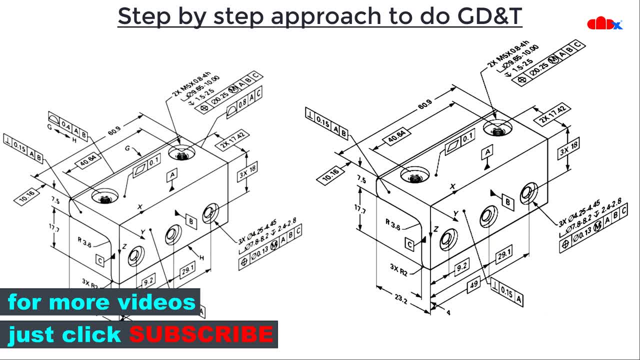 Your drawing. So this was The step by step Approach To do GDNT For any drawing. And this was The second part. Now, in third part, I will explain How to place The datums And to place 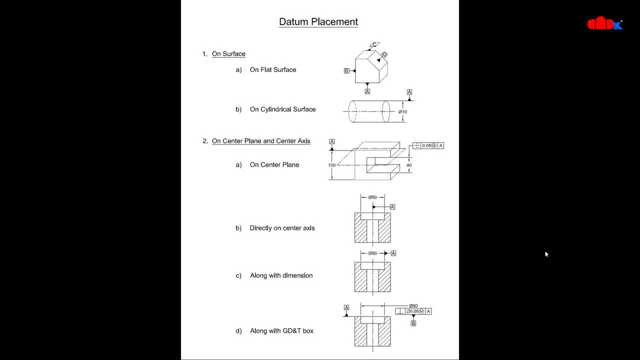 The GDNT. So let's move To the third part. And to explain The third part, I have this PDF With me Now. here You can clearly See that There are two different ways To place the datums. 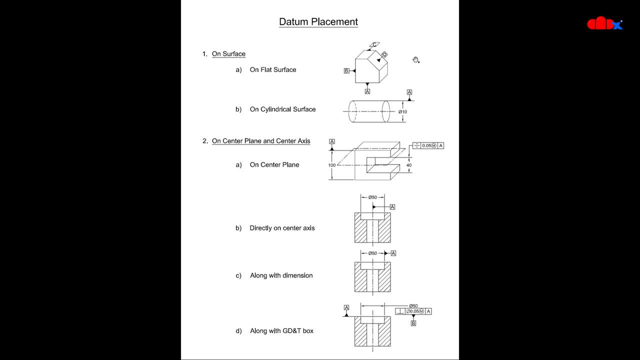 Either on surface Or on center, So you can place Your datums Like this Datum A, B, C, D. You can have multiple datums For flat surfaces. You can even apply The datum Directly. 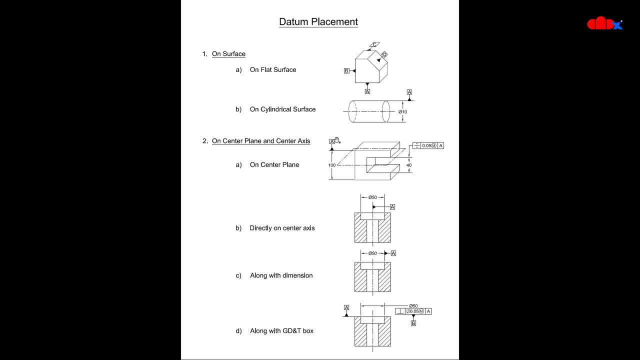 To the center plane Or center axis. So whenever A datum Is aligned With a dimension, Then you are telling That The center Of this dimension Is the datum A. The imaginary Center plane Is considered As datum A. 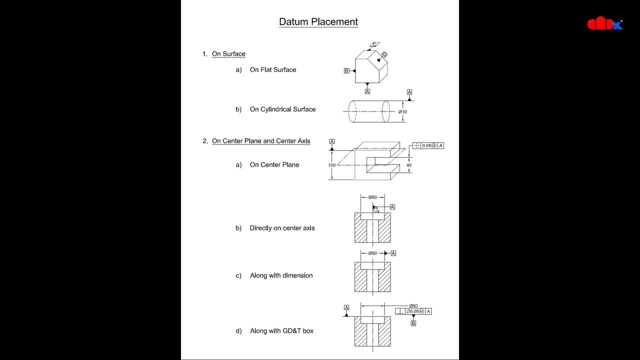 And if you go For center axis, You can directly Attach your datum To the center axis Like this, Or you can align Your datum With dimension. This also shows That this datum Is applied To this center axis. 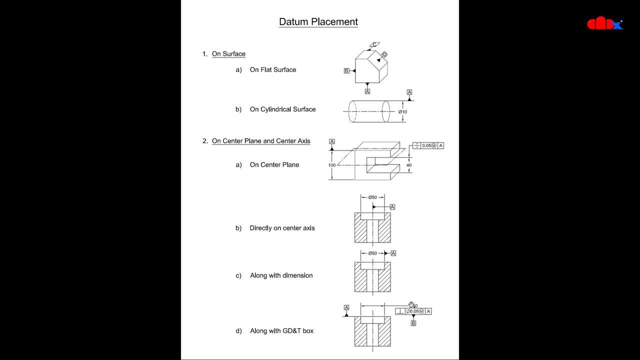 Not to this surface Or The GD&T box Which is attached With The dimension. Again, You are telling That This particular datum Is This center axis. Now here, Datum A Is this top surface, But datum B. 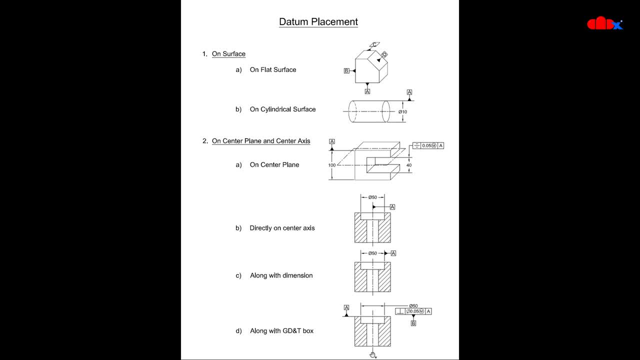 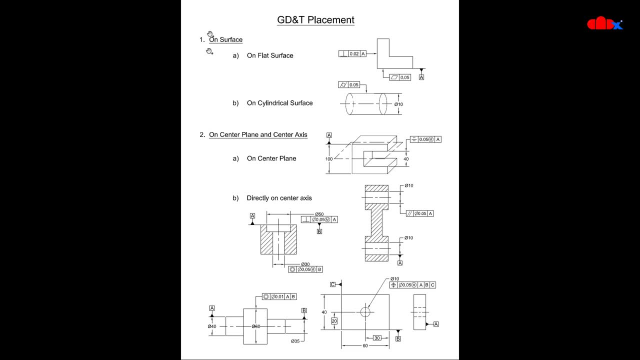 Is This center axis. So this was The two ways To place the datums In your drawing. Now let's see The GD&T placement. So again, The GD&T placement Is also done On surface Or on center. 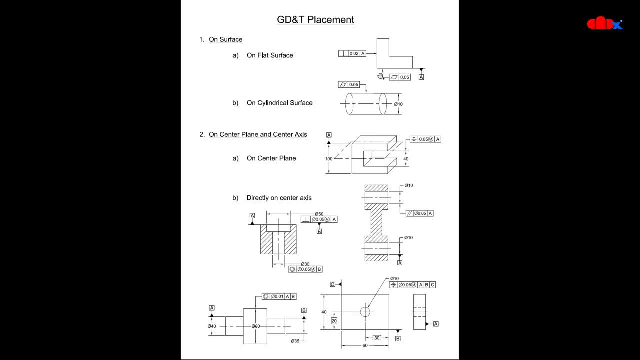 So, as On surface, You can Directly apply To the surface, Just like this, Just like this. And As On center, You can apply To center plane Or center axis. So in this case, This GD&T. 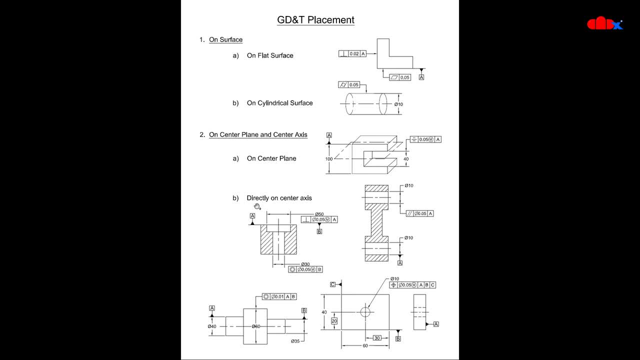 Is Applied To the center plane Now if you come down Directly On center axis. So if you understand This GD&T box, It is telling That perpendicularity Within this range, With reference of A, So the datum A. 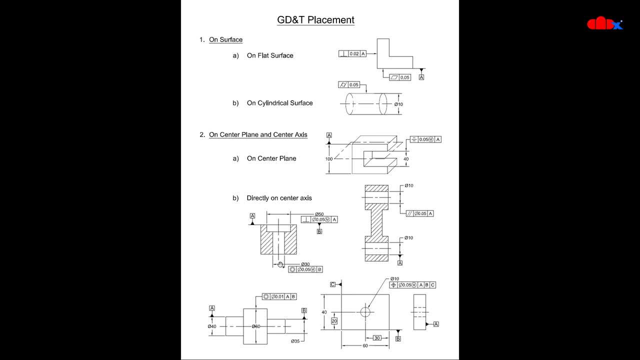 Is the top surface And datum B Is this center axis. So This GD&T box Is controlling This center axis. The center axis Has to be Perpendicular. That means It has to be 90 degree. 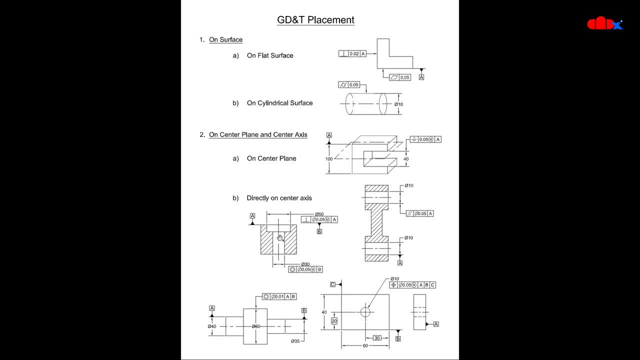 With datum A, With this top surface Within this range. So the center axis Deviation Will be Within this range. So, again, As it is applied To the dimension, It is applied To the center axis. So these are: 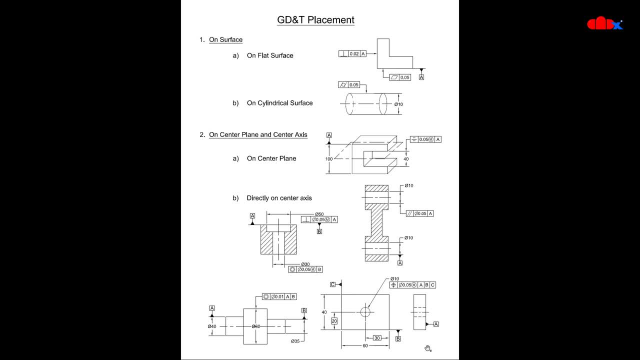 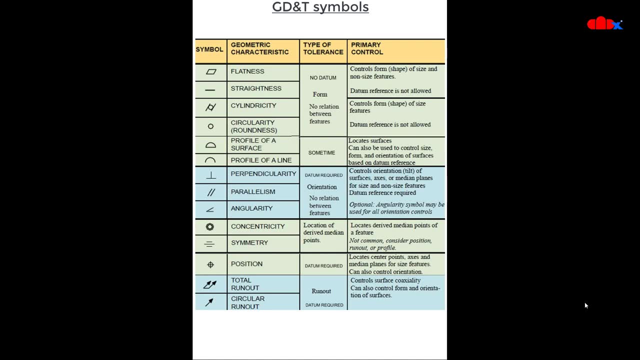 The two ways To place The datums And place The GD&T Inside the drawing. So this was The third part. So in fourth part We will understand These symbols And abbreviation. So I will start with. 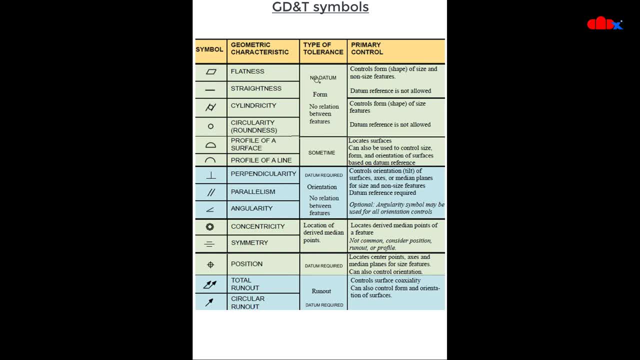 These four symbols. These four symbols Doesn't require Any datum. This control The form. Now, if you see The flatness And cylindricity, Practically Both are similar Because When you have A flat surface, 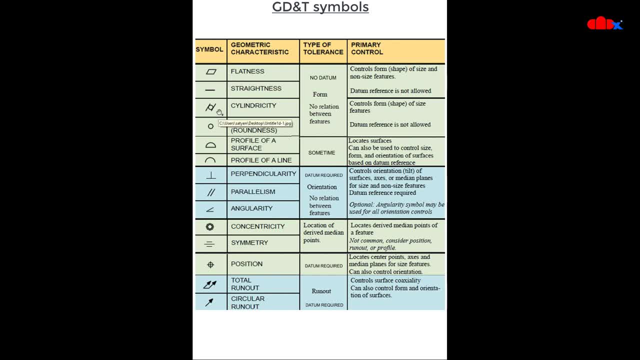 To be controlled, You put flatness, And if the surface Is cylindrical, Then you put Cylindricity. Similarly, Circularity And straightness Is having similarities. Now You can use The throughout profile Of any part. 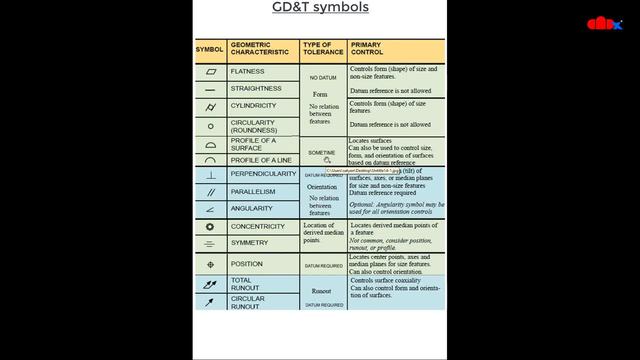 These two Also doesn't require Datum, But sometime, If it is reference With something, Then you may need The datums. Then you have These three symbols Which control The orientation, And These three symbols Are always reference. 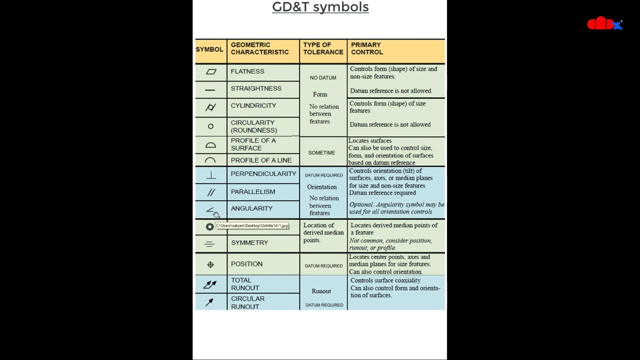 With The datums. So When you say One surface To be angular, Then you must define One more surface From where You need to Measure the angle. Then These three symbols, These three symbols Are for location. 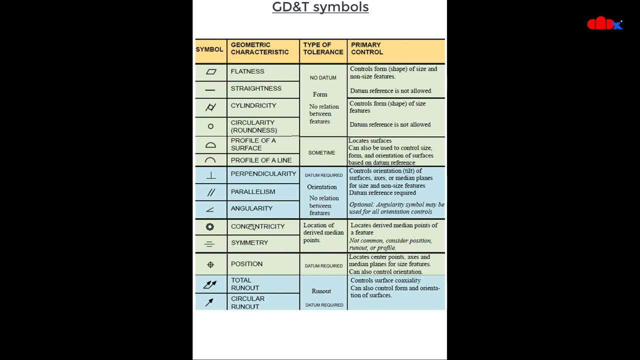 These three symbols Also require Datum, Concentricity, Symmetricity And position. At last You have two symbols Run out Which again Require datums. So these symbols You understand Little bit And once. 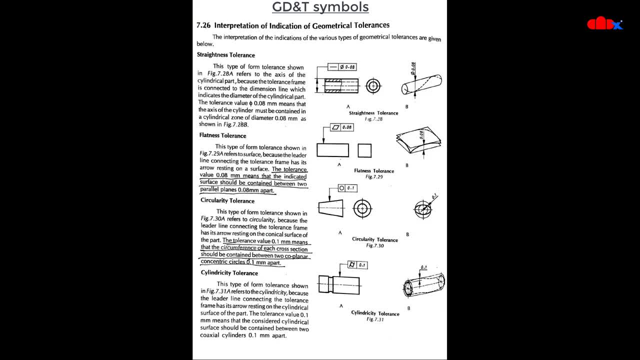 You start Working on it, You will understand Thoroughly. Now These are The abbreviation. Now, If you go for Straightness, So If you zoom This top Surface, There will be Some kind of 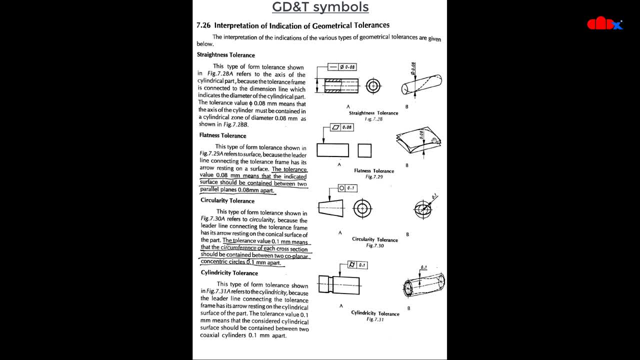 Deviation, Which is Shown here In two surfaces, And The deviation Should be Within this range. That is The range Of the top surface. If you see Straightness, If you zoom This area, 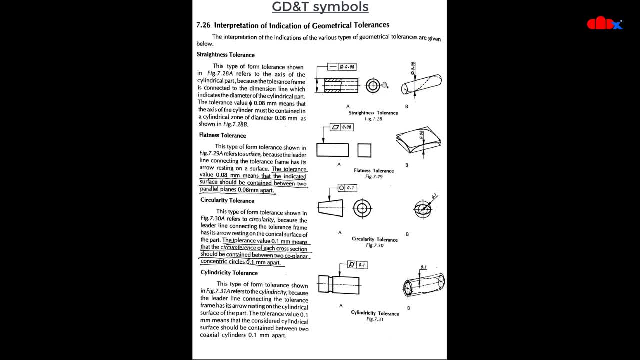 There will be Some deviation In a straight line Manner, So that Two lines Are shown Like a cylinder, Here Again Coming here, And The deviation Should be Within that Two line range. Similarly, 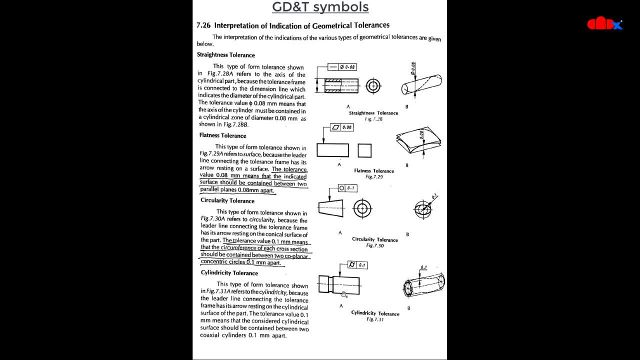 For circularity, The deviation Of the surface Within this range. Then You have Cylindricity Again. You can see Here The Cylindricity. There are Two Cylinder, One. 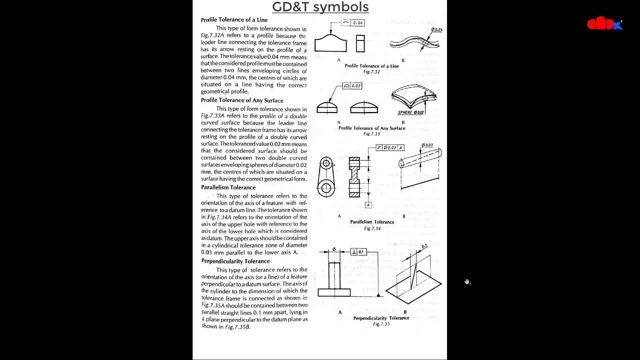 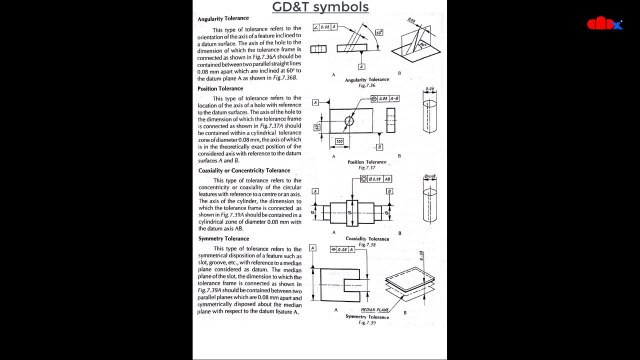 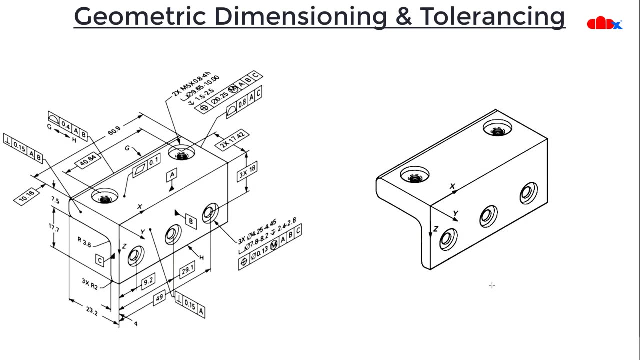 Cylinder Is This Cylinder And The Cylinder Is This Manner, Same As In the Slope Of Scenery. And This Is The Length And The Line.